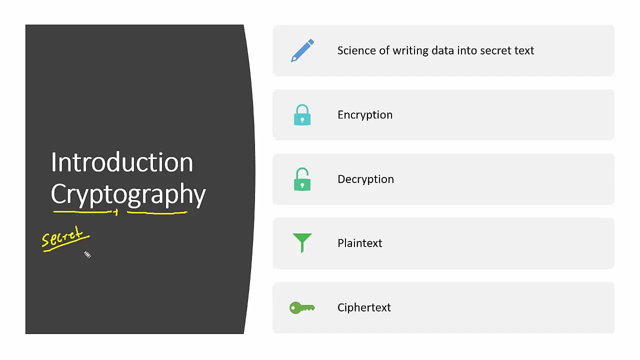 in Hindi And those who don't know Hindi. for them it's a secret, But those who know Hindi they can. those who know Hindi, they can able to understand what I said. So for the people who are not a Hindi listener, they will not able to understand, And my goal is to make 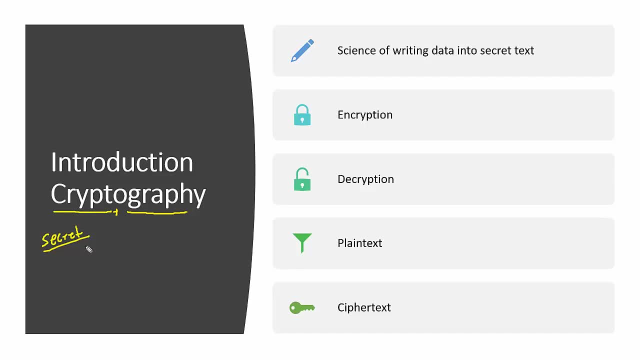 sure that this information only available to the authorized user. I spoken in the language which can only known by Hindi, So this is called as a secret text and coded test, unreadable data, And graphy is called as a science of writing science. 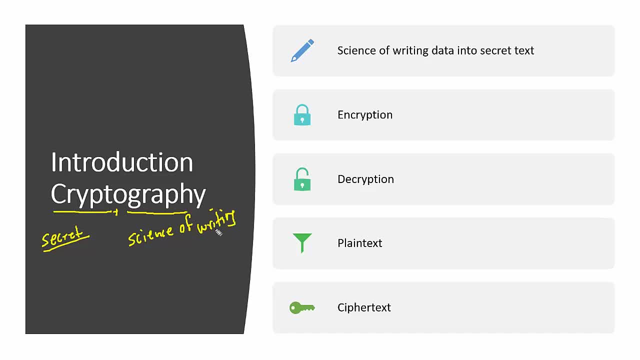 of writing. That's why, if you see the definition, it's a science of writing data. science of writing data into secret text is called cryptography. Now, in cryptography we have some basic terminologies. The first terminology is called as encryption. It means it is a process itself which convert the data from plain text into the unreadable. 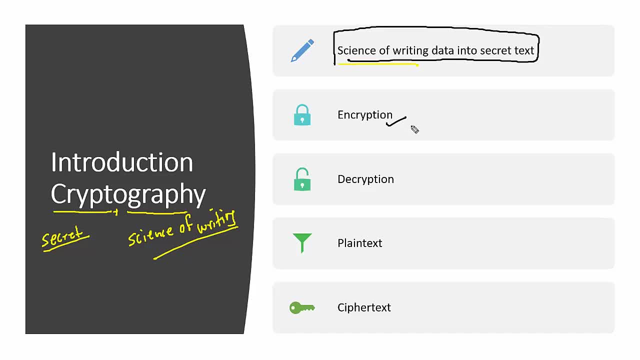 format which is only and only available to the authorized user. As I said, this is me, which is Prabh, and this is my friend, whose name is Manish, My best friend. You can say like that. He is my lovable friend. So I always use this example. 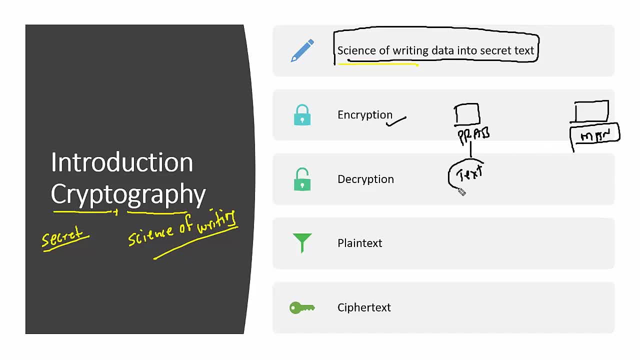 So what I did? this is my text we have, And now we have some set of 70 people here. They knows English only. So what I did? I convert this text, which is an English text, into Hindi And I told Manish: Manish bhai, I am sending you some data. 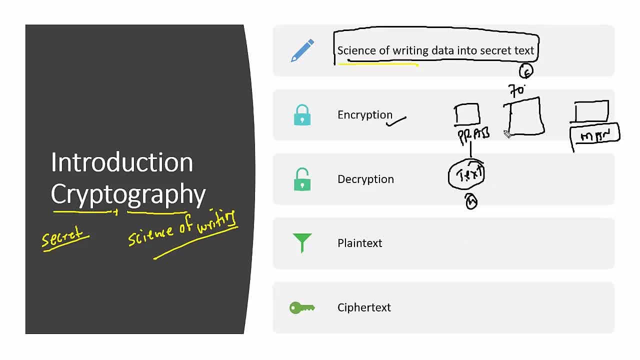 And I mention in Hindi Because if I pass through this To the 70 people, they will able to understand. So I convert it into Hindi. So when you receive, you read that, So you will get to know what I want to convey. 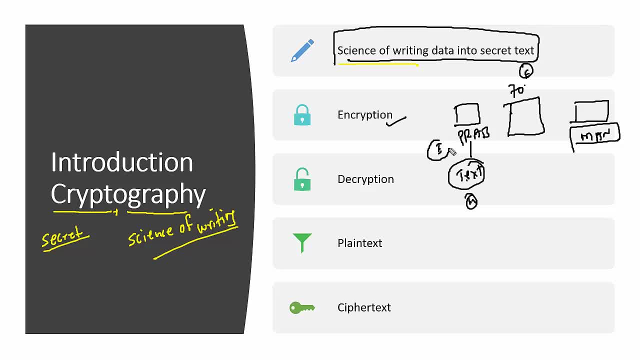 So what I did here is I convert the English into Hindi So that only Manish can able to understand This process is encryption Okay, A technique by which I convert English into Hindi? So from the information security point of view, you can say like that: 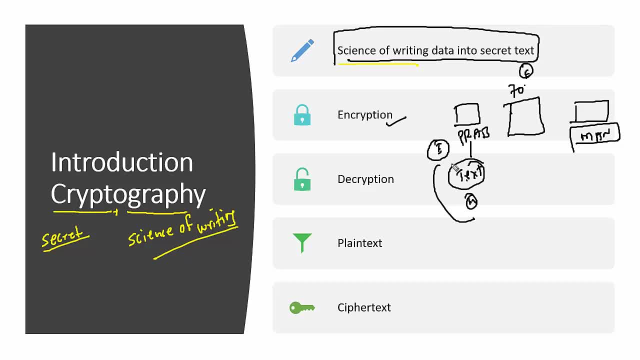 It is a process by which I convert the readable data into the unreadable format So that only authorized party can able to access. In this case, Manish can only able to understand Because Manish know in that group Hindi. But the decryption is a reverse process. 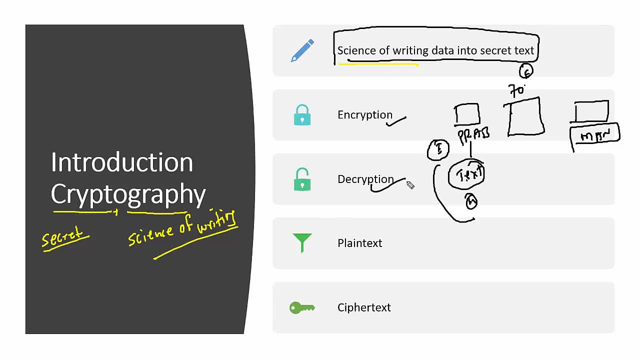 Where we decrypt the encrypt text or unreadable text back to the plain text, The representation of the readable value. that is called as a plain text. Here English was the plain text And encoded value- unreadable data. that is basically called as a ciphertext. okay, so this is the 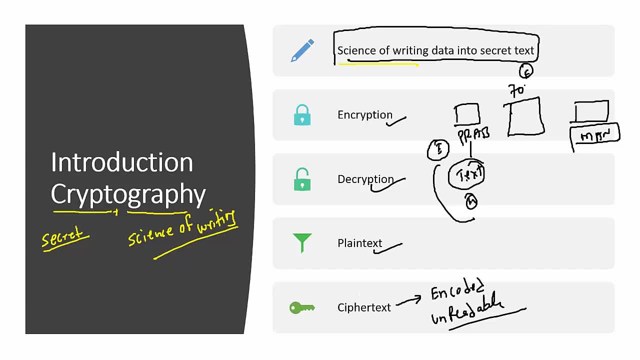 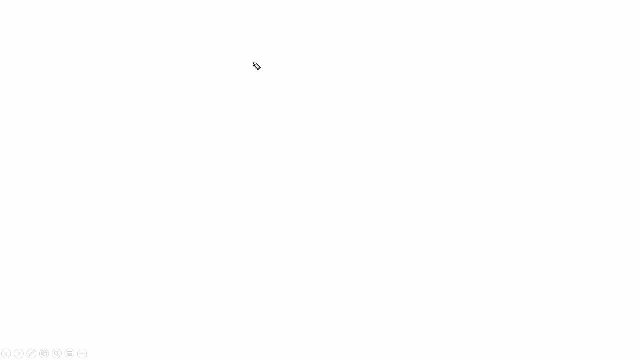 high-level process or terminologies that we used in the cryptography. now, before moving ahead, let me give you very basics overview of entire element we're going to cover now. if you take example here, if I say cryptography, crypto plus graphy, it is actually divided into two part. we have a modern cryptography and we have a 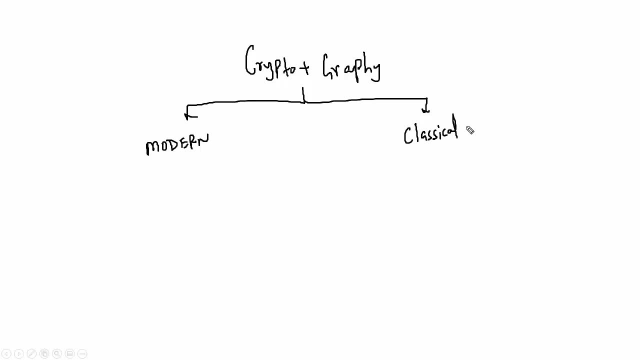 classical cryptography. if we're talking about the modern cryptography, we have a two type of modern cryptography. one is called as a symmetric and one is called as a asymmetric. but when you're talking about the classical cryptography, the classical cryptography is basically two type. one is called as a substitution and one is called as a transposition. actually, 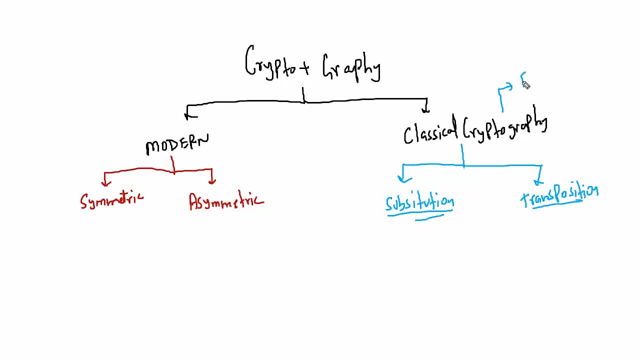 classical cryptography is more like an encoding concept and modern cryptography is more like a core encryption. now let me explain you the thin line difference between encoding and encryption. also now, when I say encoding, this is my text. we have example. this is my text. money: this is my plain text. I use one encoding language. I convert M. 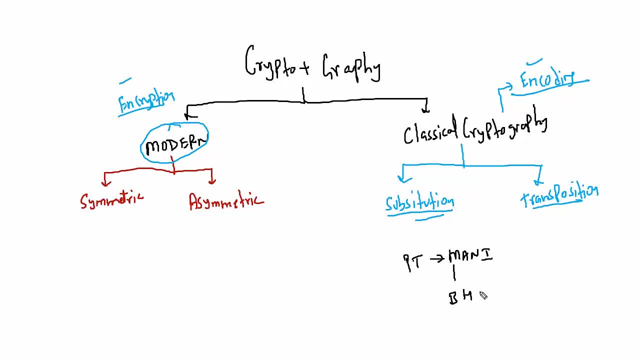 into B, I convert A into H, I convert N into D and I convert I into A. but so I replace a character to character. that is called encoding. but in the encryption what happened is we have a plain text called money and that will be convert into binary then. so this is my plain text. now we need a key. key is the logic. sorry, key. 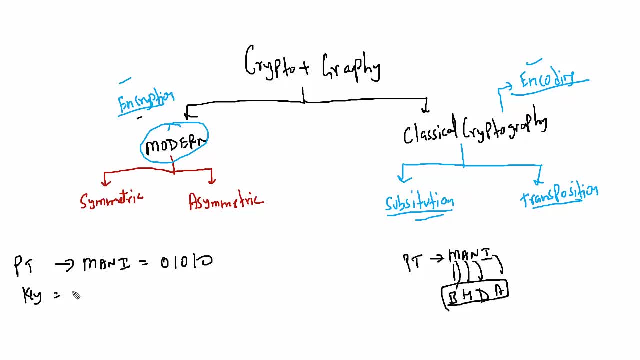 is the factor. so key is, like a passcode, capital, P, a dollar, dollar W, 0 out the example which will be convert into binary. then between that we do the ex Mitar just giving an example and that value will be my cypher text value. that is why encryption take more time than encoding. encryption take more. 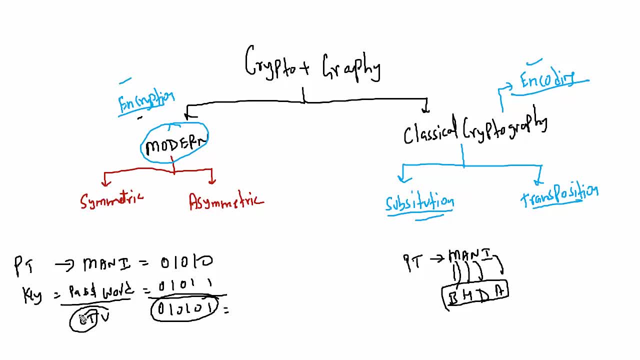 processing, then encoding. so we we are doing a changes in the binary level in the encryption, where in the encoding we are introducing a changes in the character level. Coming back to the cryptography part, in cryptography we have a two important component. one is called as a key and one is called as a algorithm. one is called as a key and one is called as. 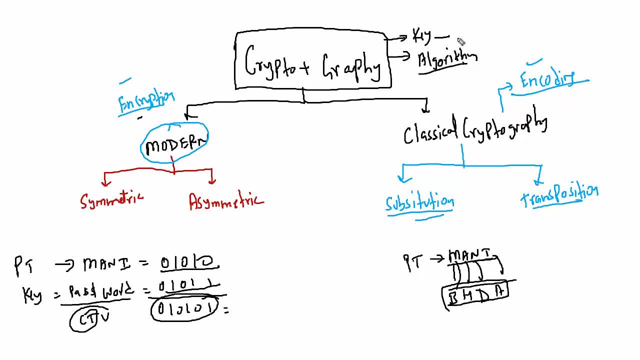 a algorithm. So key is called as a factor and algorithm is called as a logic. Let's take example one, and logic I use plus. I am using one base language here which is like a alphabet: A, B, C, D, E, F, G, H, I. 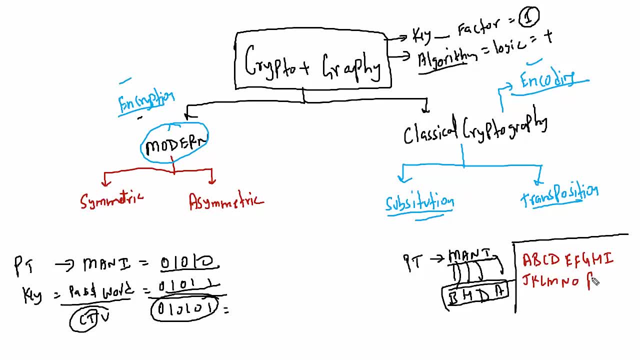 J, K, L, M, N, O, P, Q, R, S, T, U, V, W, X, Y, Z. So this is the alphabet diagrams. So when I using a classical cryptography, what I did, I use key as a one and plus as a logic. then I combine that plus one because algorithm. is called as a logic: b, c, d, e, f, g, h, io, p, q, l, m, n, o, p, q, r, s, t, u, v, w, x, y, z. So when I use in a classical cryptography what I did, I use key as a one and plus as a logic. then I combine that plus one, because algorithm is called as a logic. 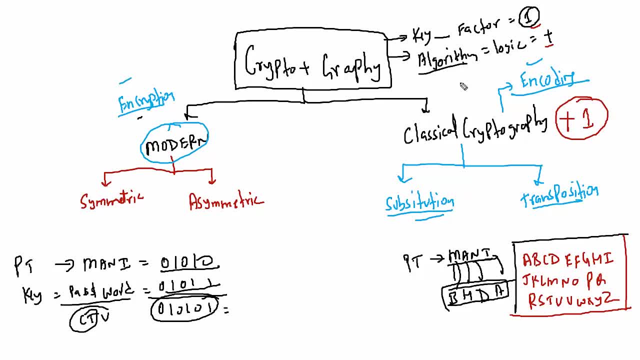 algroupz az happened, for we used crucial in new meaning. So algorithm is called as a logic English. I'm using as an algorithm, but by why? but what is the phrases I'm using in an English to communicate? that is called as a key because key is the factor. I will show you the example now. in the substitution: 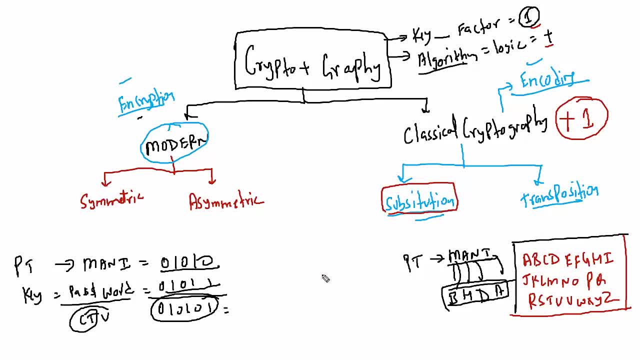 cryptography. what happened is? this is my plain text, called let me delete that. okay, now I have a plain text which is called security. okay, this is my plain text, and now I want to encode a text. so what I did? I use a plus one. substitution mean using an. 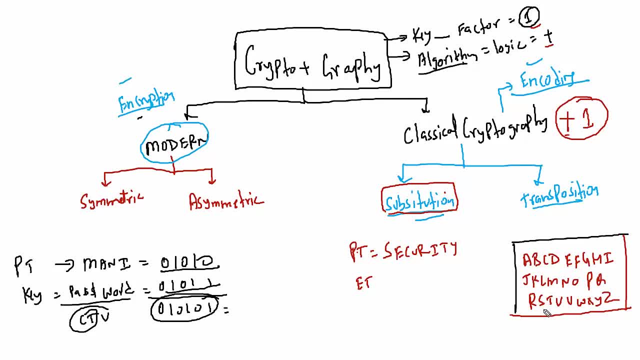 alternate value. so we have a s, s. that is SS, s, plus one is T, because s after s plus one is coming as a T. so I use the T as a value: e, e, e, plus one is F, C, C, C, plus one is D, u, plus one is R, R, plus one is s, I. we have a I, then we have a J, then we have a T. we. 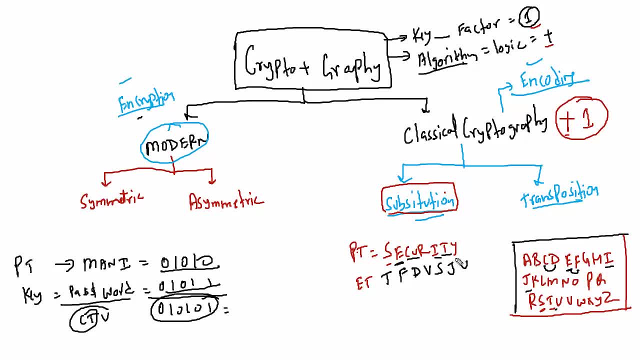 have a T, U and Y Y set. so this is basically my encoded text. if you notice, if the key length is small, it is easy to find the pattern. now, instead of plus one, I use minus. one example: so we have s. we have s, s before minus R. so this: 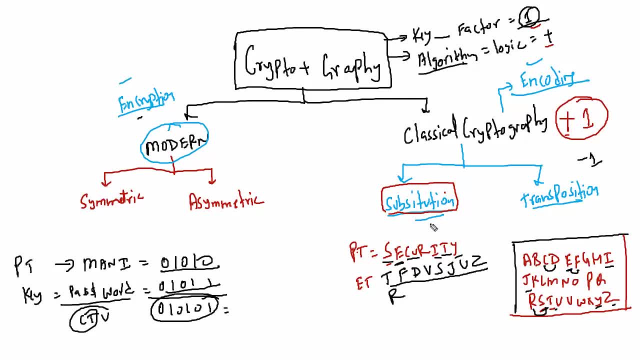 will be the R. so in substitution we finding an alternate word. but when we talking about transposition, transposition mean trans plus position, transparently. we changing the position. transparently, we changing the position how s plus one is e, so e will be the first. e plus one is C, C will be the. 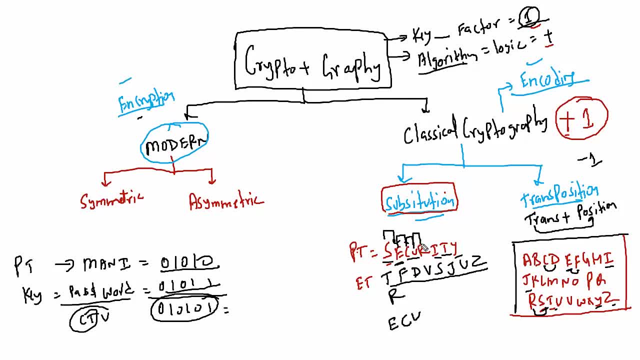 second C, plus one is u, u, u, plus one is c. c will be the second c, plus one is u, u, plus one is R, R, plus one is I, I, plus one is T, T, plus one is Y, Y, plus one is s. so this is how I use the transposition cipher. okay, in substitution, we finding an. 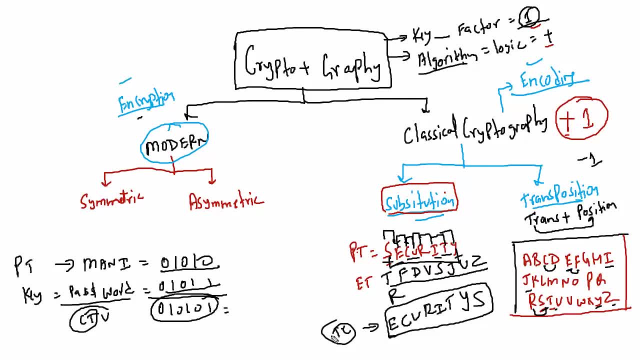 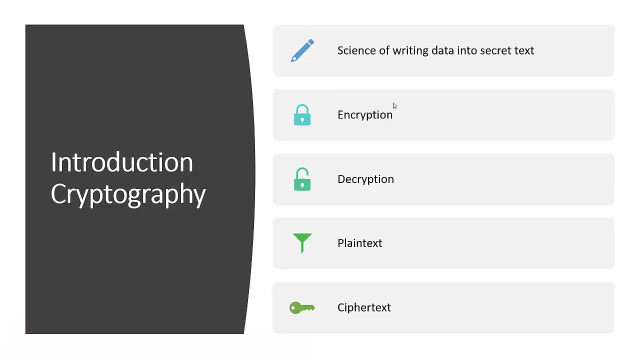 alternate word, but in the transposition we finding the. we just replacing the character. so this is the high level summary of classical cryptography, but what we going to learn in modern is a symmetric and asymmetric. in my next slide now, when you talking about cryptography, as I said, encryption, decryption, plaintext and ciphertext in 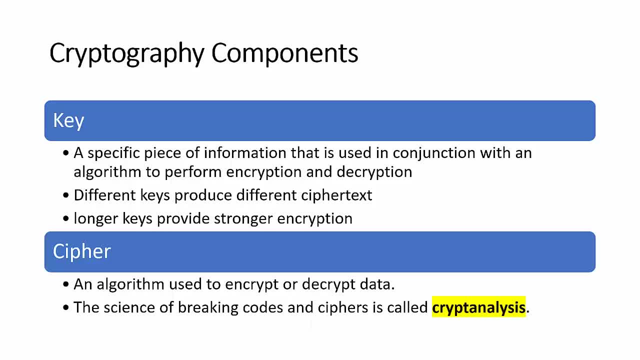 modern cryptography. we have a two major components: a very, very important, which got enhanced. one is called as a key and one is called as a cipher. another name of the cipher is algorithm, so key is a specific piece of information that is used in a congestion with the algorithm to perform the encryption and 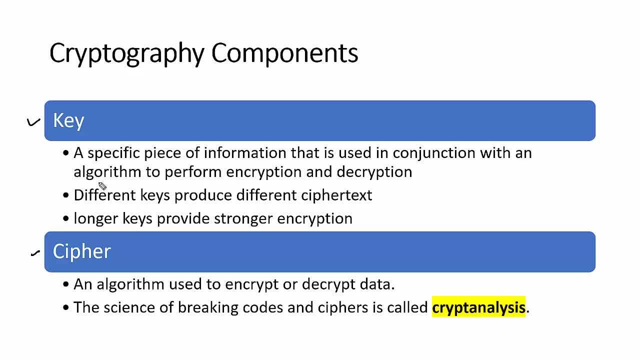 decryption. if you saw in my previous example, plus and one. so plus was the algorithm and one was the key which is used together to perform the encryption and decryption. I told Manish a, Manish a, plus one is B, so remember. so plus is the algorithm, calculation with alphabets, and one is basically the factor. so one simple. 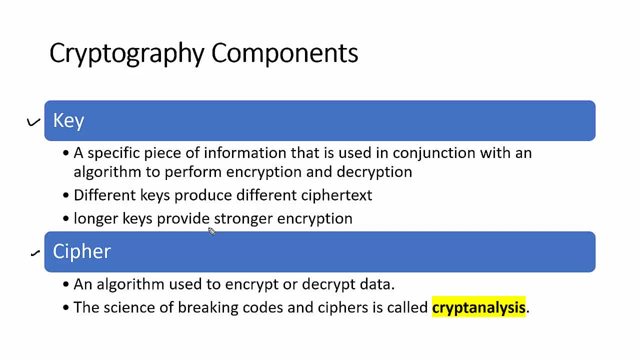 rule you need to remember is that you need to remember that you need to know the key with reference to the key. longer key produce the stronger encryption. let's take example: my key length is one, one, one one, so it will produce the fixed output of one one, one example. but if I have a larger key, plus two, three, five, six, seven, 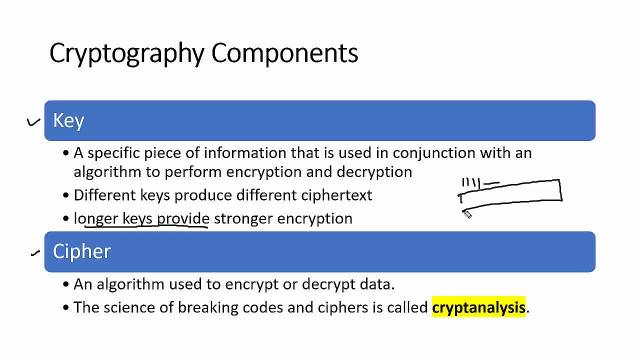 so they will see that two, three, five, six pattern and by which they basically form the key. that's why we say: larger the key or bigger the key, more secure and more stronger will be the encryption output. told manish, okay, remember, uh plus 73. so then they will calculate the plus 73 values and then it 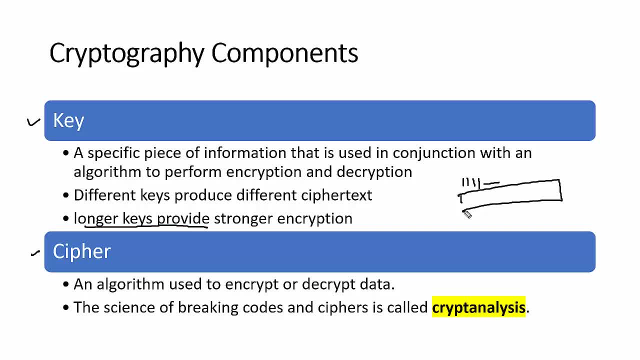 produce the output. but problem is that bigger key, higher key, bigger key size will produce the more secure output, but it take more time also. so whenever we selecting the key for the encryption, okay, we need to balance the performance and security. that's why we called as a key is the. 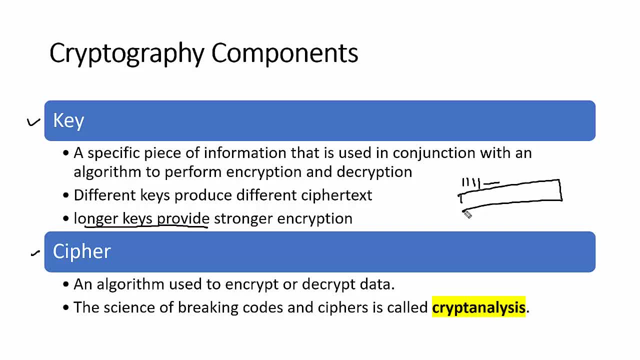 process which is used with algorithm to encrypt and decrypt the data, and cypher is called as an algorithm. another name of cypher is algorithm, which is used to encrypt, decrypt the data, and there is a process called science of breaking the code or learning the cryptography algorithm, or 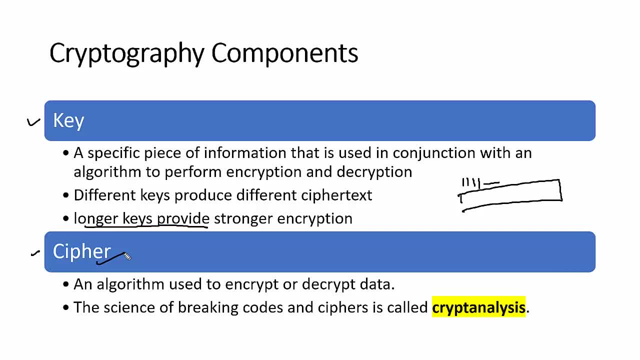 finding a weakness and that process is called as a crypt analysis. a lot of company higher crypt analysis whose primary role is to discover the weakness in the cryptography algorithm, study the cryptography system, so they can able to break it. now there is a possibility, like me running a cryptography solutions. so what i did? i hired the cryptography professionals and i told 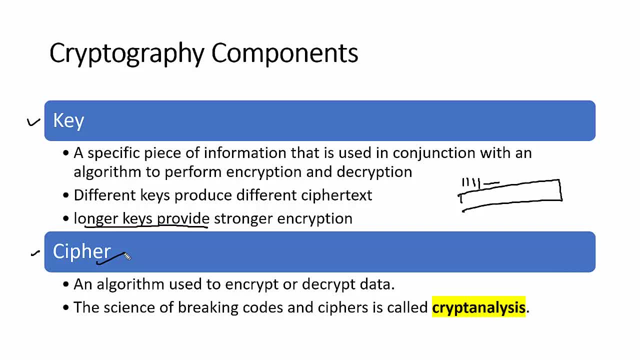 them find the weakness in my system, find the weakness in my algorithm. so they tried to break my algorithm. how the data which is encrypted by the algorithm. they try to break the data, they try to recover the plain text from the data and then they will give me the report. okay, by this. 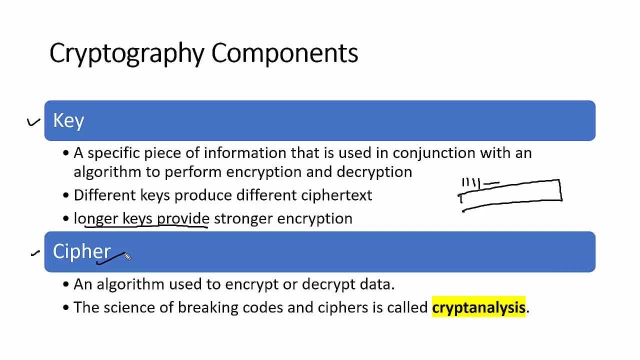 factor, we able to break it. so we will add that information to the algorithm and then we will add the information and make the algorithm more secure. so, study of algorithm, process of breaking, that is called as a crypt analysis. moving to the next part, we're going to cover about type of 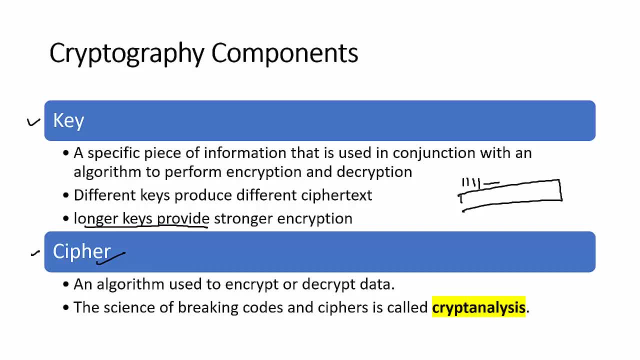 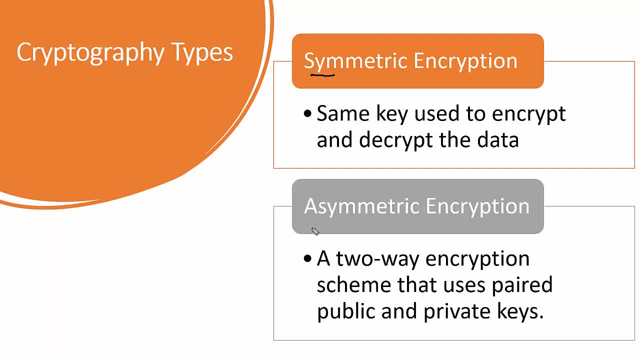 cryptography, which is called symmetric and asymmetric. let's move to the next part. okay, so symmetric encryption and asymmetric encryption, if you go by the description. symmetric- key used to encrypt and decrypt the data. symmetric: use the same key which is used to encrypt and decrypt the data. that is called symmetric. 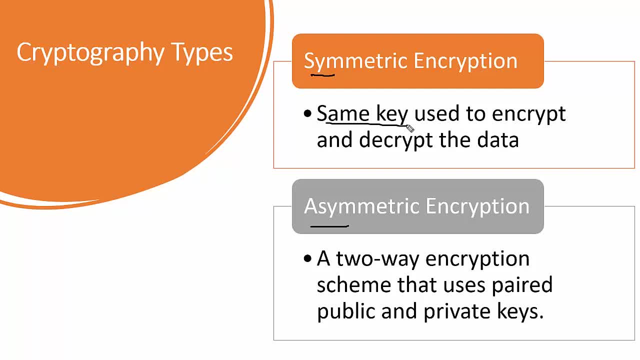 encryption and asymmetric is basically used two-way encryption that is used with pair, public key and private key. it means one key is used to encrypt and one key used to decrypt. okay, so how it works, let me explain you. so let's start with the first part, which is called: 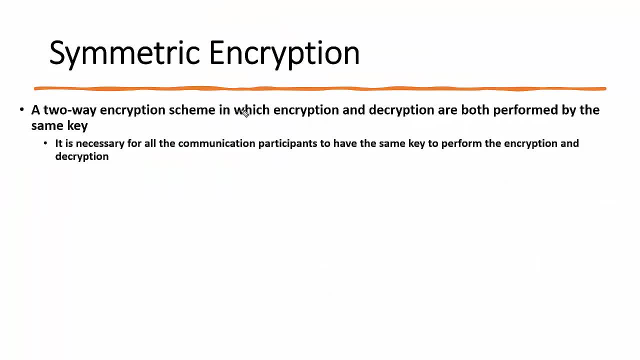 as a symmetric encryption. so if you read the description, it is clearly say that two-way encryption scheme in which encryption and decryption are both performed by the same key. okay, so the first part is called symmetric key. how? let's take example, we have a system a and we have a system b. this is my data. 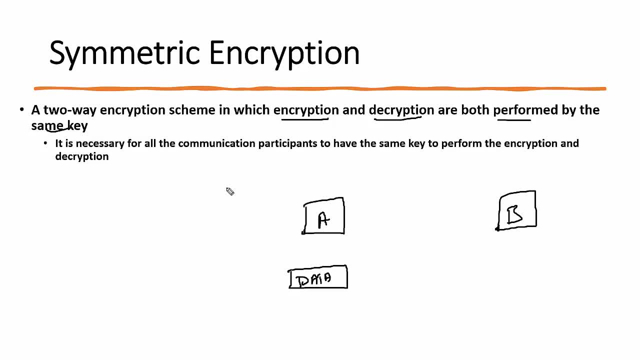 so we got one key which is called as a. this is called as a symmetric key. now we have a different name for that. we call symmetric key, we called session key, we called secret key. okay, we called private key. have a different name. or in your language you can say: this is a password. you can say: 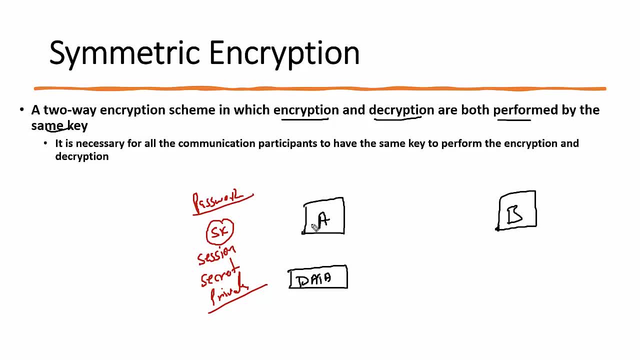 like that. in a very layman term, it is called as a password. so what i did? a basically use his key plus algorithm to encrypt this data and produce the cipher text. the same example i have shown you. it is same. like you know, you have a winrar document and you protect the window document. 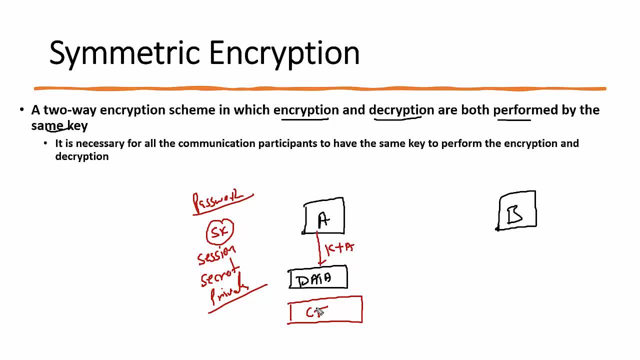 with the password, right, so here the password is called as a key. okay, so key is suppose: uh, one, two, seven, nine, eight. so this is the key we have, which is used with the algorithm to encrypt the data, and this is the cipher text we produce, which is called as unreadable data. 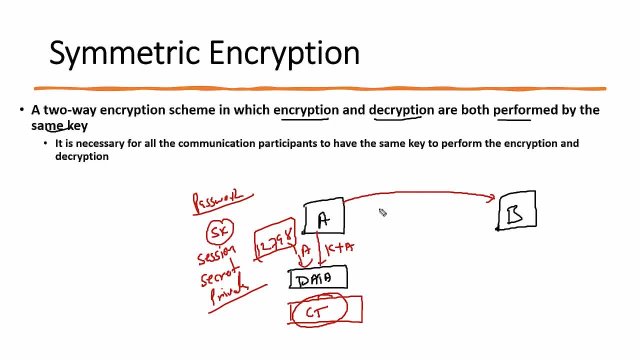 now a sent this data to b. okay, it is a encrypted data which is sent to be now be received. the encrypted data same like if i protect the file with my password. you will ask for the b and you could create a password for certain partner data apps. 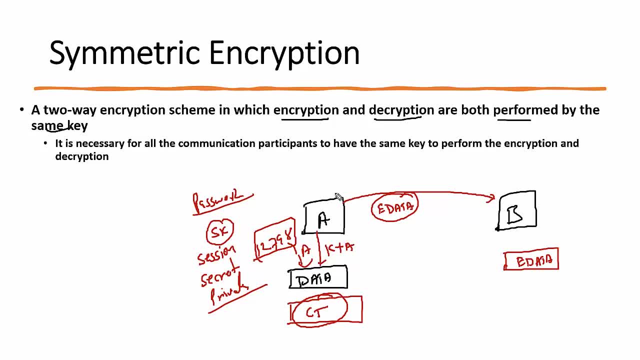 ask for the password only now. concern here is i have to send my key, the same key, so i sent 1, 2, 7, 9, 8. so be applied: 1, 2, 7, 9, 8, by which? and plus algorithm and decrypt the data. 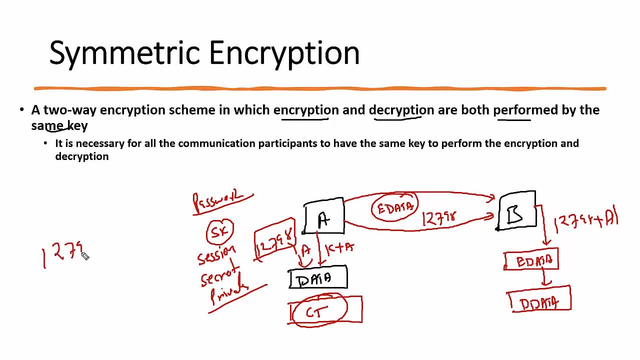 okay. so that is why we use 1, 2, 7, 9, 8 to encrypt the data and to decrypt the data. that is why today's symmetric encryption is used for the data encryption today, if you take an example of aes- you heard about aes on your browser- wireless aes- they all are symmetric. 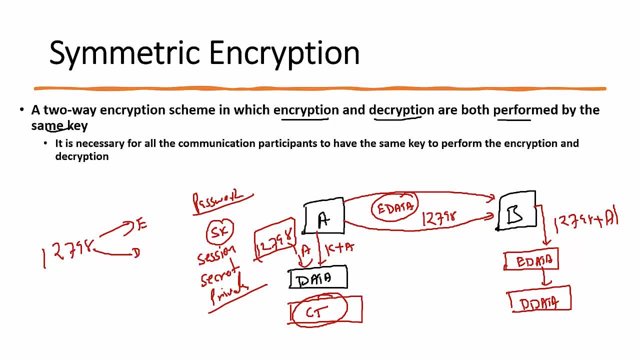 encryption only where we using a same key to encrypt and decrypt the data. now there is one concern here. the concern is: if you sending the data and key in a same channel, this is called as the same channel. now what happened? there is attacker, he can intercept the encrypted data also and he can 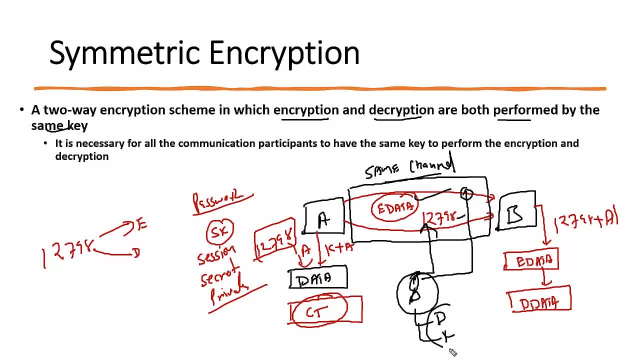 intercept the key also. so by this way he get the data also and key also. so that is why the biggest concern with symmetric encryption is the key exchange. key exchange and that is why they use multiple technique. one is called oob, out of band. it means sending a key by email, sending a key in a hard disk, sending a key in. 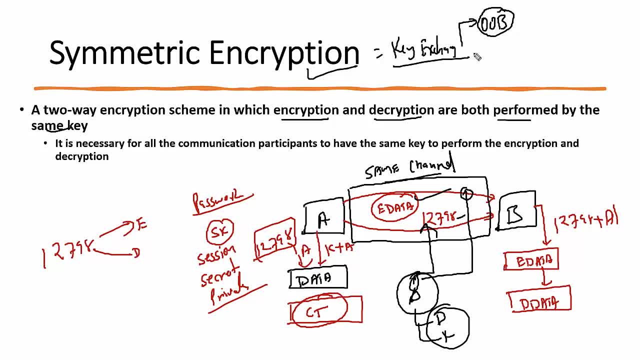 a pen drive or calling the person and dictate the key, or the second process. they will use asymmetric process that i'm going to discuss in the next slide. so the primary concern with symmetric encryption is the key exchange, but today, primarily symmetric encryption is used for encrypting a data because it is faster in processing the data, because same key used to. 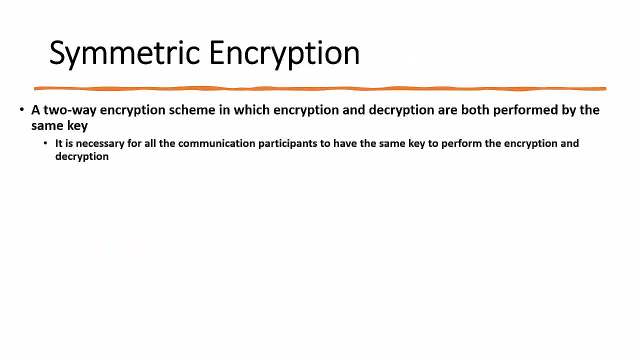 encrypt and decrypt the data. so when you document symmetric encryption, we have a two type of symmetric encryption. one is called stream based and one is called block based. now when i say stream base, example: youtube: okay, so in stream is what happened? whatever the data we have, it is convert into binary. 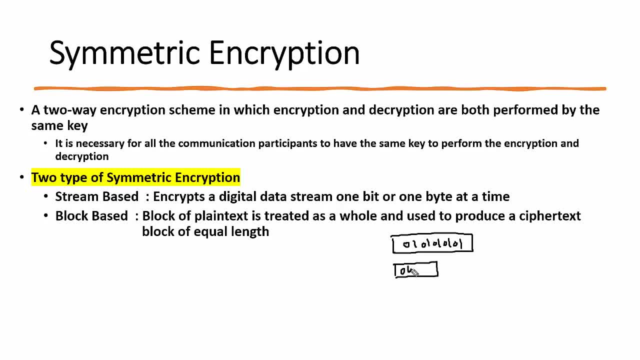 and whatever the key we have. okay, it is also convert in the binary. so in the stream based encryption it encrypt the digital data stream one bit or one byte at the time. it mean they do like a this way. so bit by bit stream is basically happen. example in my video: if 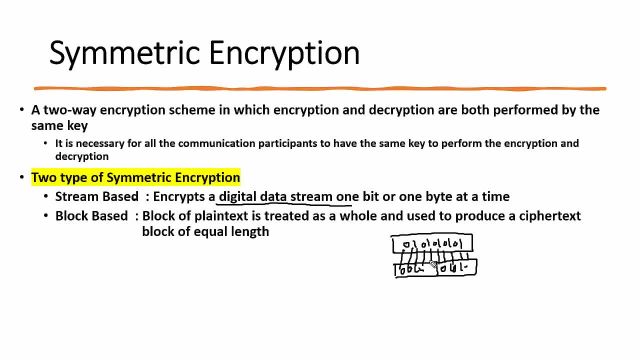 if I upload this video on a YouTube and you playing my video, okay, with, smoothly, without any interruption, thanks to the using a stream based encryption, okay, they encrypting bit by bit parallelly. okay, bit by bit parallelly. okay, bit by bit parallelly on a same time. so that is called as a stream based encryption. but 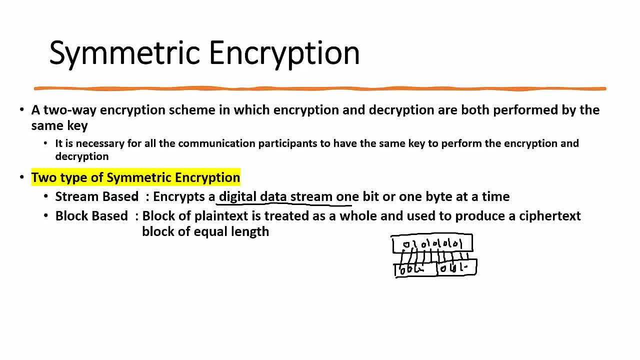 when we're talking on block base in block base. what happened? we have a data here, data divided into block one, block two and block three, and then each block is basically encrypt by the same key and then we send this block. now, if YouTube is using a block based encryption for the video streaming, 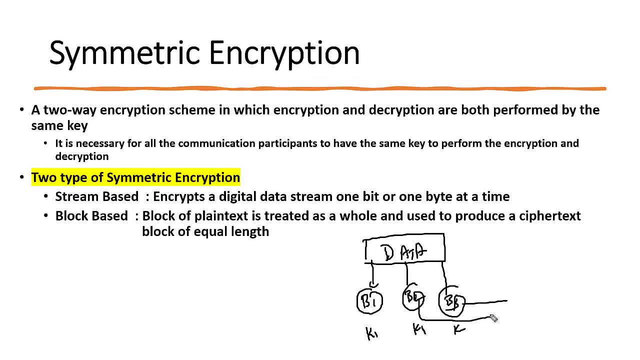 you can see that it is using a block based encryption for the video streaming. so my voice will be like that: hey guys, is that clear or not? so, if you see, these are some interruptions, because data was not something parallelly getting encrypted, decrypted. it is not something parallelly going bit by bit encryption. 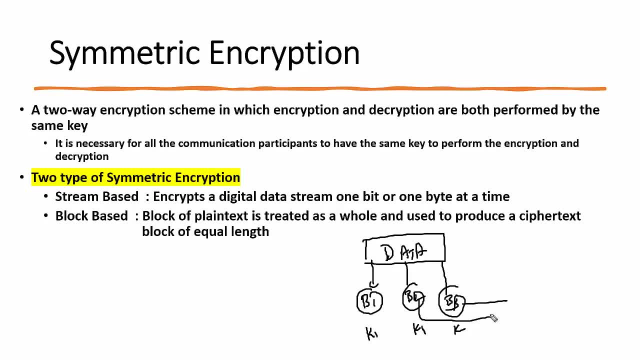 data divided into block and each block is basically encrypted by the keys. that is why block based encryption use in that case when data resides somewhere in a storage. okay, so stream base use an application, block base use in a hardware. so these are the two type of encryptions we have, so key. 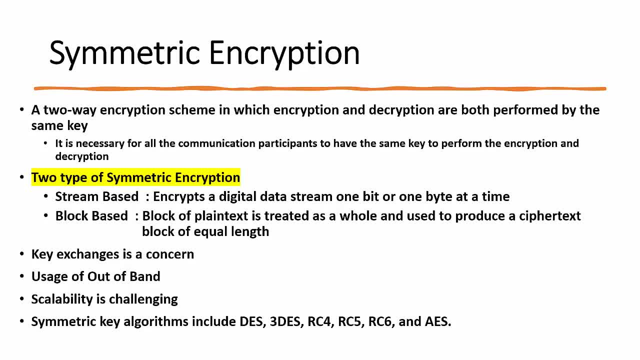 exchange is a concern because same channel we are using, so we use the out-of-band exchange. scalability is another challenge we have because for every user we need to have a unique keys. example like this way: we have a system a and we have a system B, we have a system C and we have a system D, B, C, D, I. 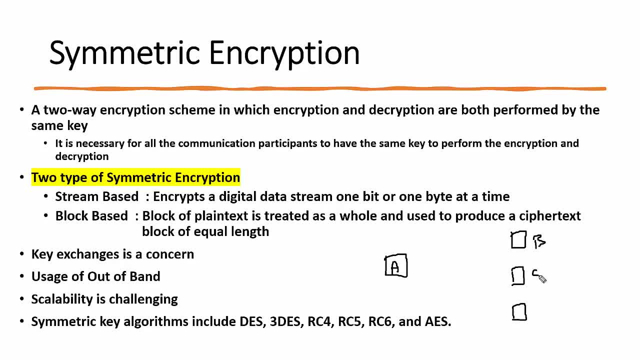 so we have a system a and we have a system B, we have a system C and we have a system D, B, C, D. for every encryption we need a unique key. so imagine more and more host now: b want to send data, he need to send his key. b need to send to c, he need to send to his key. so for every user. 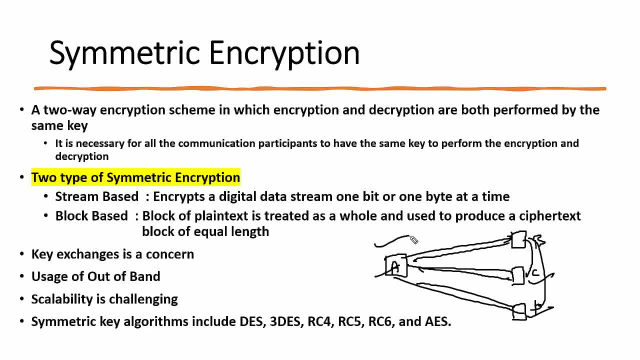 b need to issue the new keys for every user. a need to issue the new keys to every user so as more and more hosts increase, scalability become a concern and we have some algorithms which support the symmetric DES 3, DES, RC4. these are the symmetric algorithms we have. 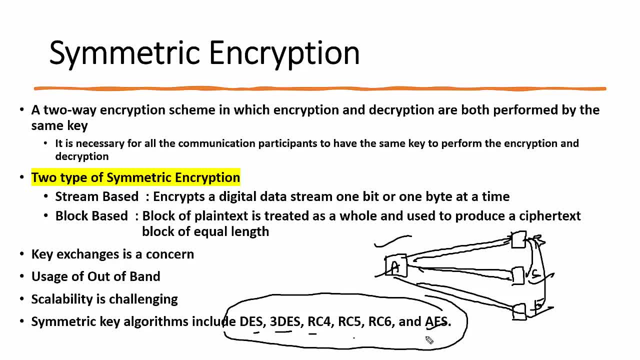 currently we using AES, which is a replacement of the DES algorithm. the biggest reason of using not using DES is it require lot of compute. and all that and AES, which is advanced encryption standard, they basically provide the better security and better functionality with better compute parameters. so that is the advantage we get when you go with the symmetric algorithm. 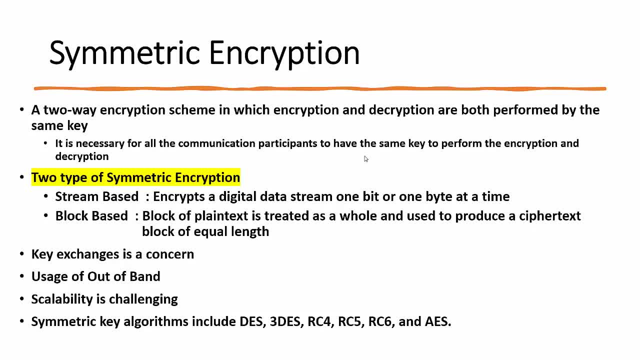 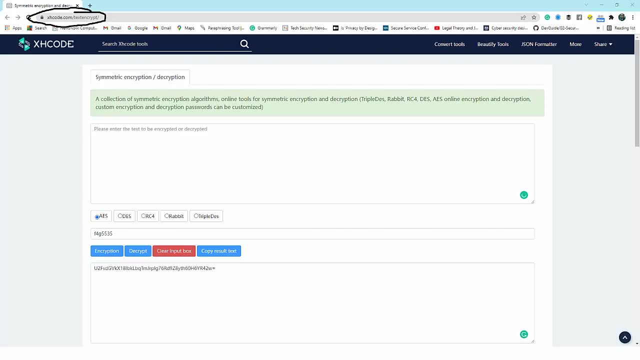 AES algorithm. sorry, so I'm sure you get the understanding of symmetric so how it works, symmetric algorithm in a real time. let me show you. let me show you, let me show you the practical demonstration of symmetric algorithm. AES algorithm is the practical demonstration. so I use this website called xcodecom, ok, 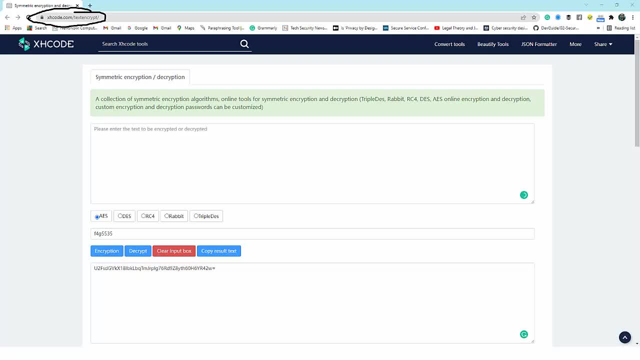 that is the name of the website we have which I used in this region. now what I did. I'm going to type the message here: hi prep, ok, hi prop. I use AES algorithm. this is the key we have that I'm using. this is the key which I'm using to encrypt the data. let me try to perform the encryption so. 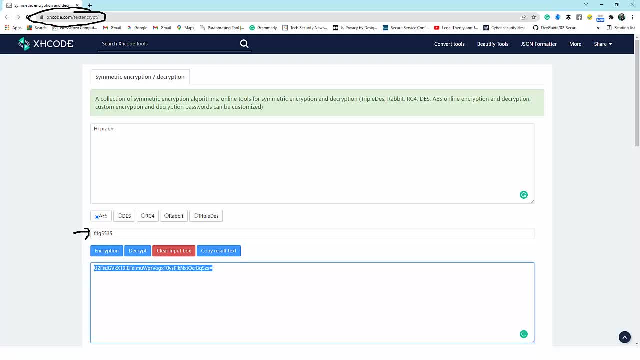 this is the cipher text we have. okay, this is called as a cipher text. so this is called as a cipher text. now what I did? I copy this and paste here. sorry, I copy this and I paste here. okay, now I'll try to decrypt so you can see hyperb. so we have used the same key we have. 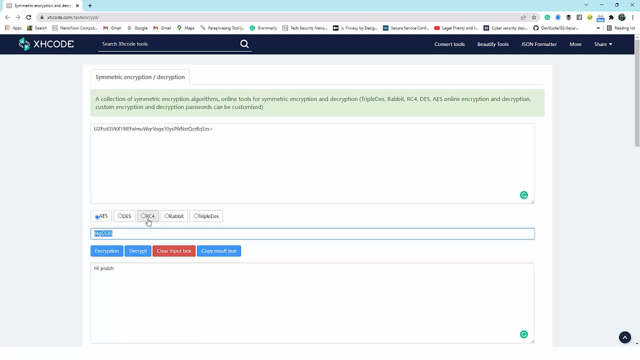 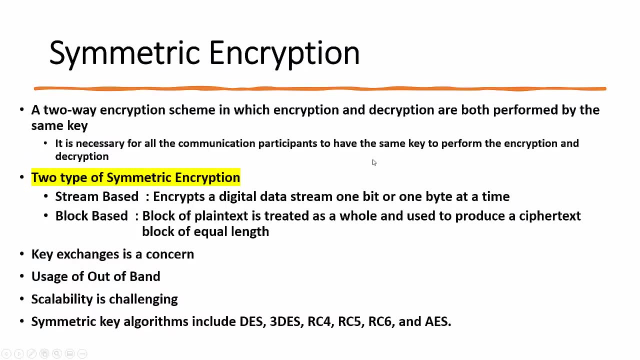 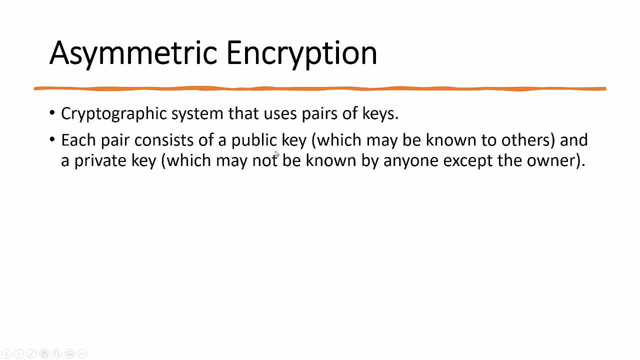 asymmetric. we use the pair of keys. each pair consists of public key, which is known to others, and private key, which is only known to the owners. so that is what is called as a asymmetric encryption. so how it works. let me explain you now. we have a system a and we have a system B. 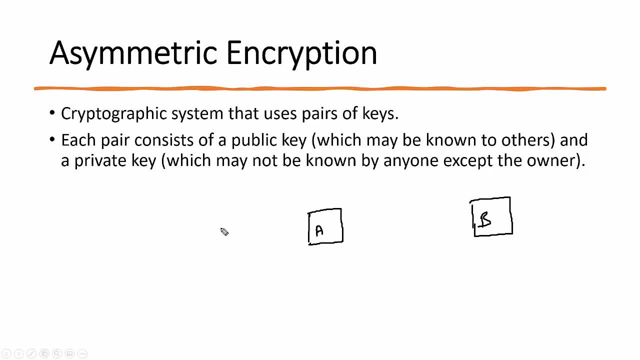 okay, so we have a public key here. let me draw it. so we have a public key, a, and we have a private key, a. we also have a public key and private key. let me draw it. so this time we have our two keys: public key and private key. so now we have a data. so this is my data, now a want to encrypt this data and send. 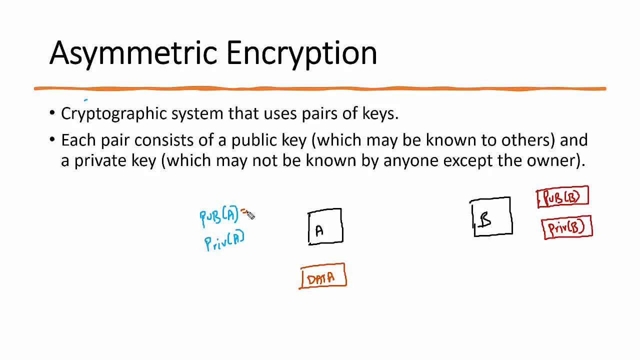 it to the B. so when I say public key, public key, something which is known to other, that what we share and private key is basically may not be known by anyone except a. okay, so a first request be public key, then B: A basically apply public key of B and encrypt the data. 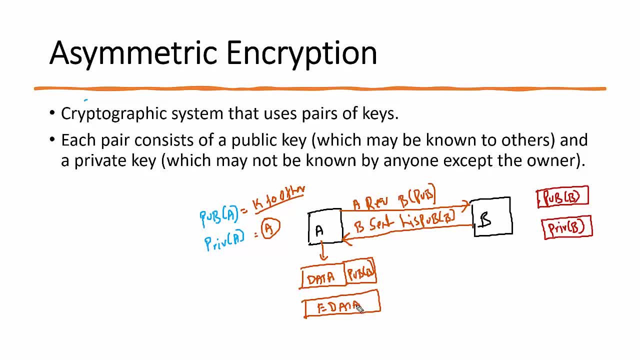 So this is the encrypted data we have, and then A send this encrypted data to B. When we receive encrypted data, he apply his private key and by which we decrypt the data. Now, if there is an attacker, suppose, if there is an attacker and he intercept from here, 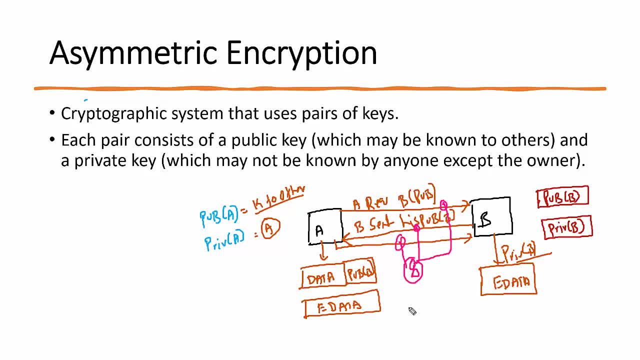 he intercept here also and it intercept here. So he got the access to the encrypted data. He got the access to the private key, Public key of B. still, he cannot do anything with that because he need another portion of a key, which is called as a private key, which we don't share. 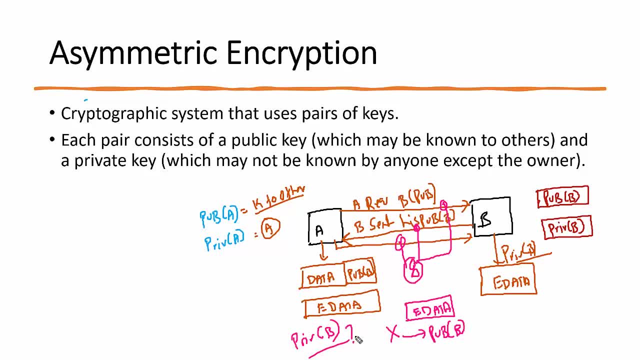 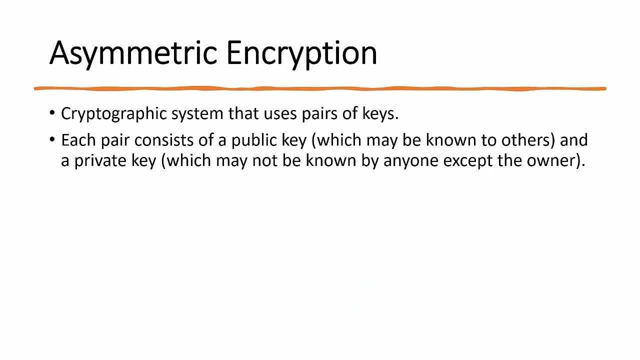 So one key is basically used to encrypt and one key is used to decrypt. So this is how it works. That's why we use asymmetric encryption to exchange the symmetric key. Let me give you that example also Now. So We have a system A and we have a system B. As I said, we have a public key A and we 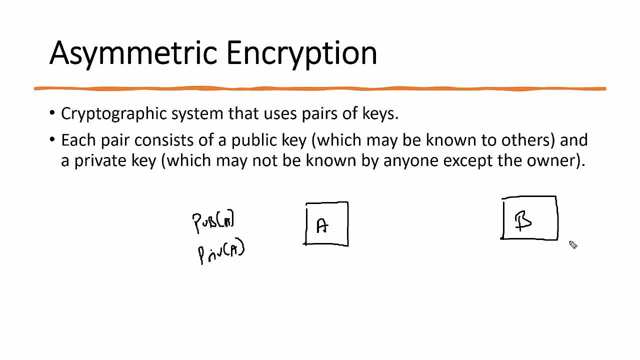 have a private key A, We have a public key B and we have a private key B. We always generate a key pair. Now we have a data. This is my data, What I did here. we also have one more key, which is called as a session key, and the name. 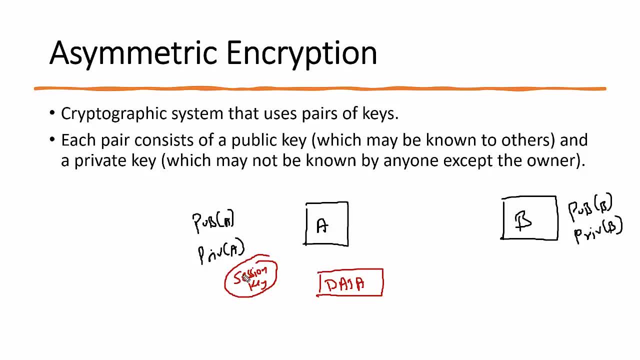 of session key is symmetric key, So now A have a three keys. Always remember in cryptography: fundamental: sender- generate the session key. sender: generate the session key. So here, A is a sender and B is the receiver. A is the source and B is the destination. 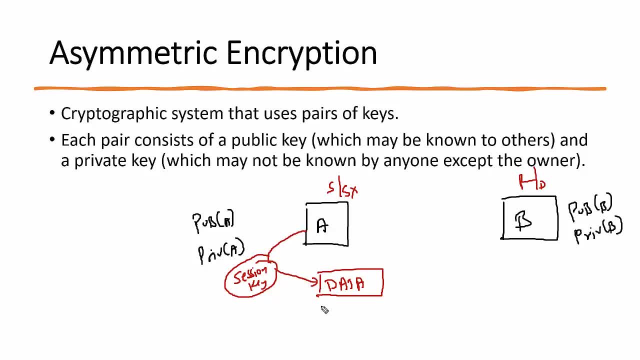 So A basically use the session key and encrypt the data. So this is the encrypted data A will send to the B. A sent encrypted data to B. Now B received the encrypted data. Problem is that now B need to decrypt, So in this case B will send his public key. 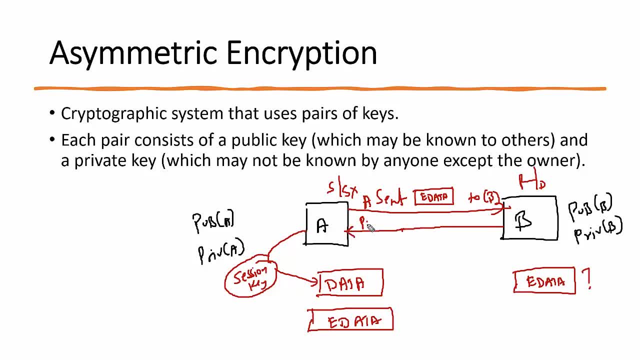 You know why? I will tell you why. So B sent his public key. The reason why: by this key only we decrypt the data, But they cannot send. A cannot send the session key over the network, So B will send his public key. 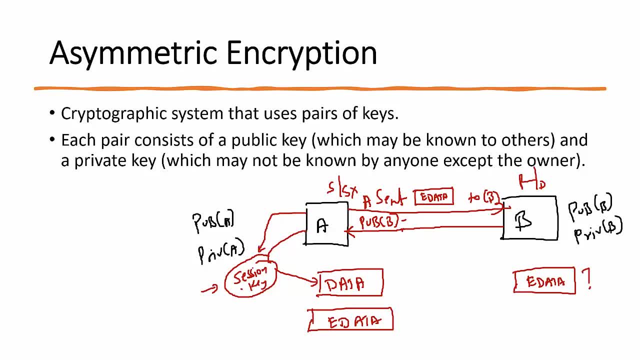 A will basically apply B public key. A will apply. sorry, A will apply B public key. B public key. B public key to encrypt the session key, because by Android session key is a value only, And then we encrypt and send back the encrypted session key to B. Now B received the encrypted. 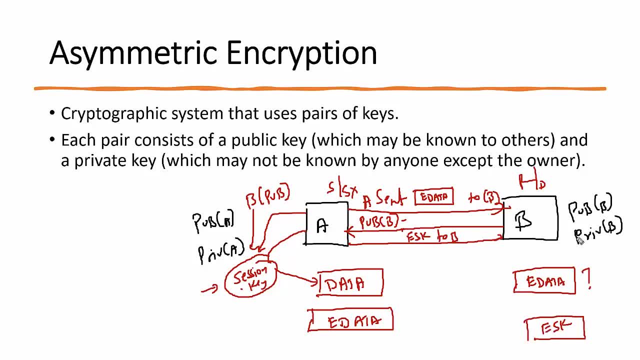 session key B will apply his private key to find the session key And then session key used to decrypt the data. That is how asymmetric is used with the symmetric. So Summary is that symmetric used for data encryption and asymmetric is used for the key exchange. 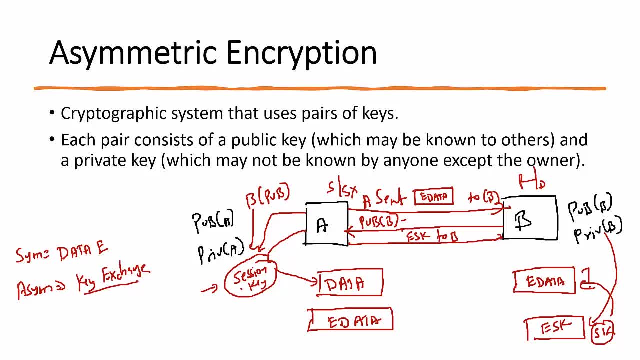 I am sure this point is clear to everyone. One primary advantage with symmetric is it is faster because we are using the same key to encrypt and decrypt. But one primary disadvantage with the asymmetric is that slow because one portion of the key used to encrypt and one portion of the key used to decrypt. 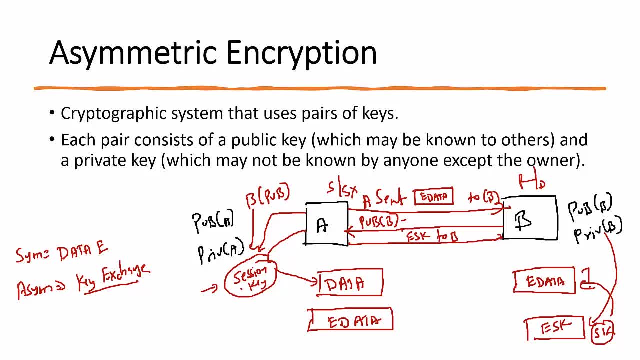 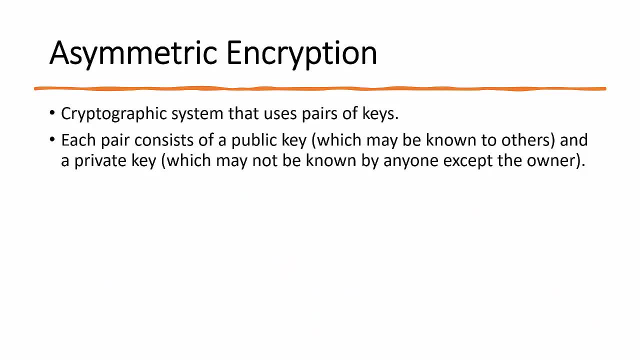 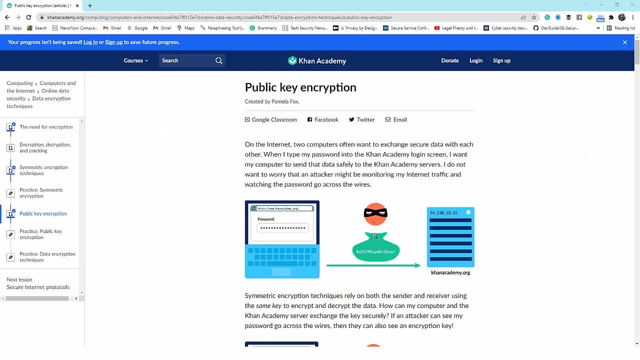 Let me show you the practical demonstration of asymmetric encryption. Thanks to Khan Academy, They did the amazing job, So I am using their website reference for this practical. Another name of the asymmetric cryptography is also called as a public key cryptography, because we are using a public key to encrypt. 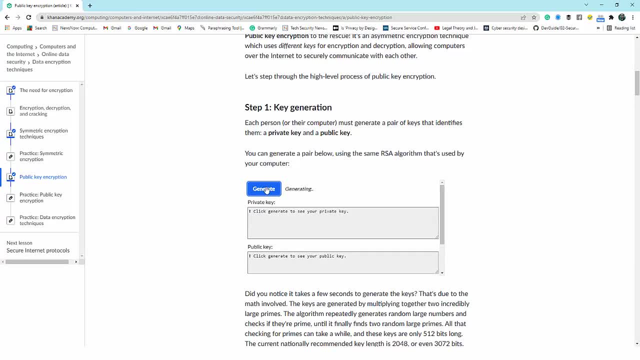 So this is the website called Khan Academy. Here we are generating a key pair- Okay, Key pair. So we generate the public key and private key. So what I did? I copied the public key And now I type a high prep. 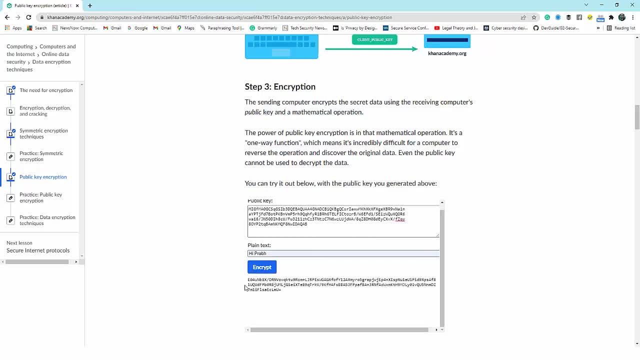 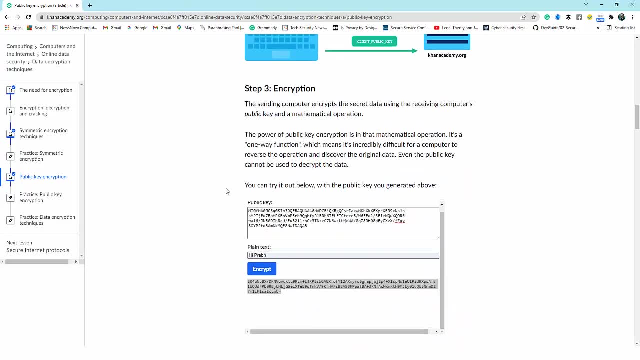 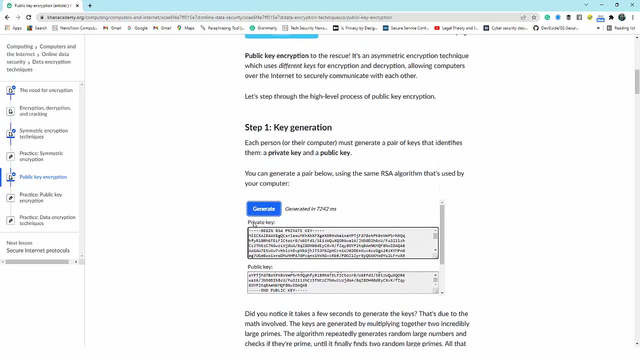 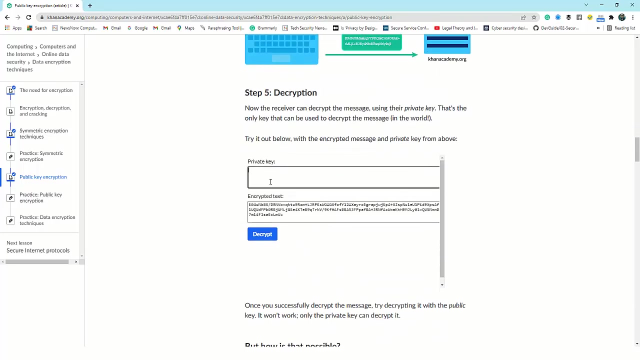 I click on the public key, I encrypt. So this is the ciphertext. we have Now what I did. I paste the ciphertext here. Now we have a private key, We have a private key here. I copy that and we have a private key. 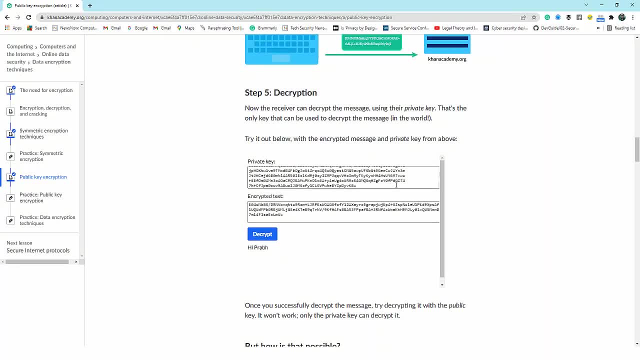 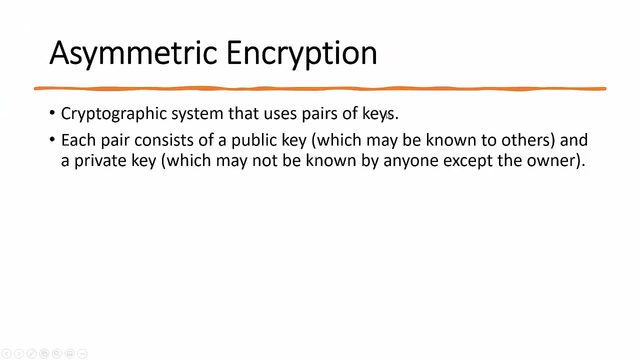 See, I got the same message, So you can see the size and all that. okay, So when you're talking about asymmetric- one portion of a key used to encrypt and one portion of a key used to decrypt- the biggest concern is performance and primary use for the key. 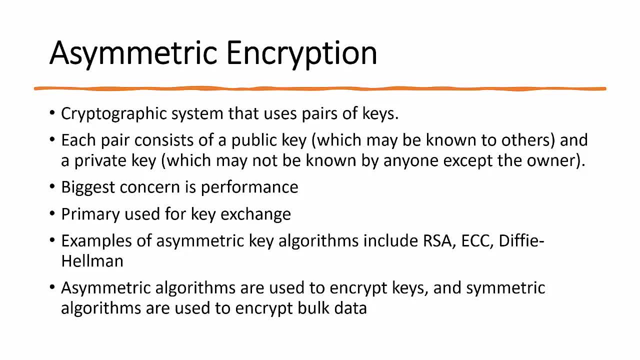 exchange. we have a different kind of algorithm, like rsa, ecc. ecc was the alternate of rsa because it take less compute to perform encryption. we have a diffie-hellman also, so asymmetric algorithm are used to encrypt the keys and semantic algorithm are used to encrypt the bulk data. so this is what. 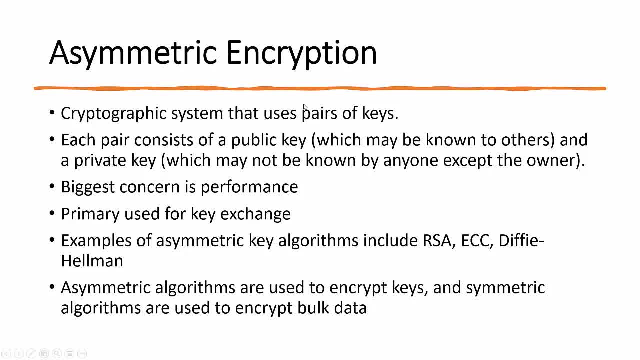 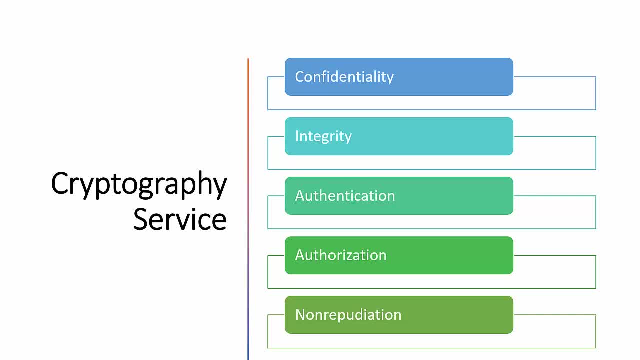 we have when you're talking about the overall cryptography. cryptography offer the confidentiality, okay. it offer the integrity where the data has not been altered in an unauthorized manner since it was created, transmit and store, how we going to discuss in my next video. it also offer the authentication by which we verify the identity of the user or system that created the information. 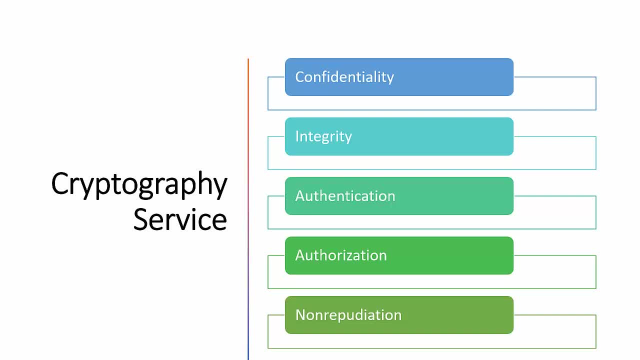 authorization. those who have a key they can able to decrypt and by this performance it able to achieve the non-reputation with the sender cannot deny for his actions. so cryptography offer: five major services with the cryptography offer. five major services with the cryptography offer. five major services with 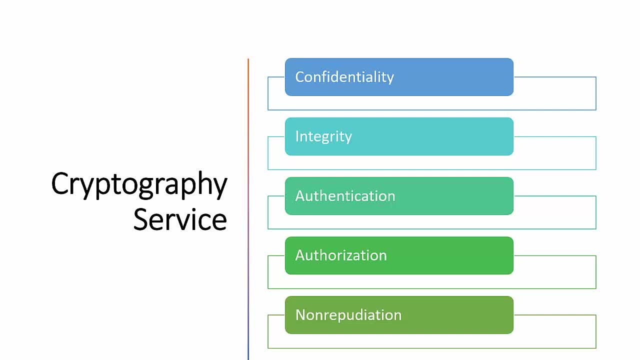 our for cryptography, we can be able to provide the five major outcome of information security. so it's non reputation, authentication, integrity we going to cover in my hashing topic, which I'm making soon. so this is all from my site and if you find this video use will do share in your 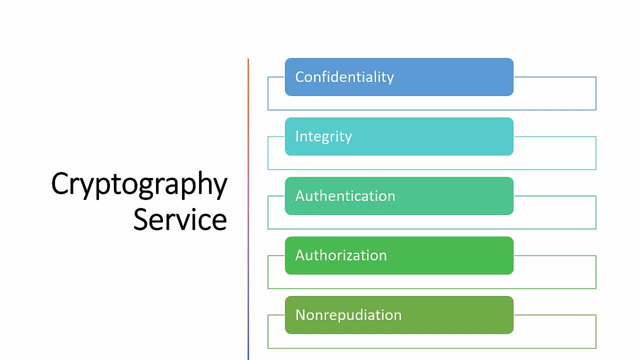 network and do let me know what is the best thing you like about this video. another important thing: I want you to do one homework and let me know what is the thin line difference between the AES and did's and ECC versus RSA and need your reply in my comment box. Thank you for watching my video.